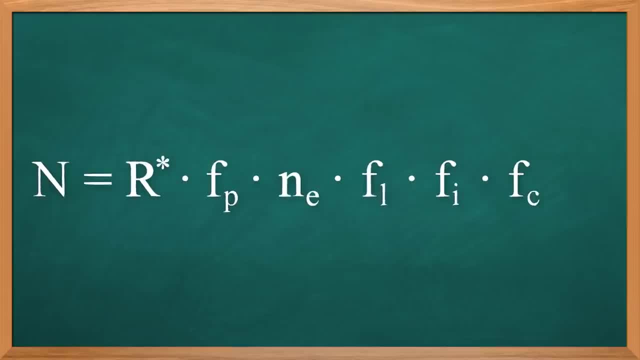 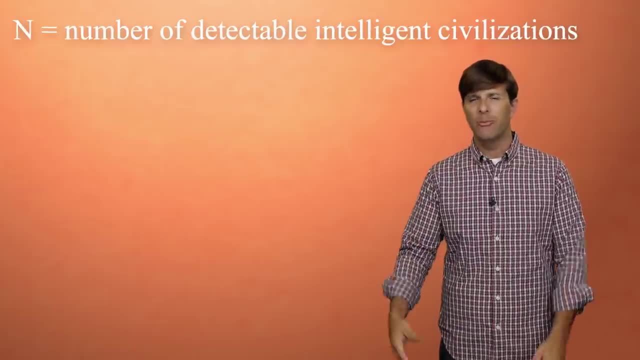 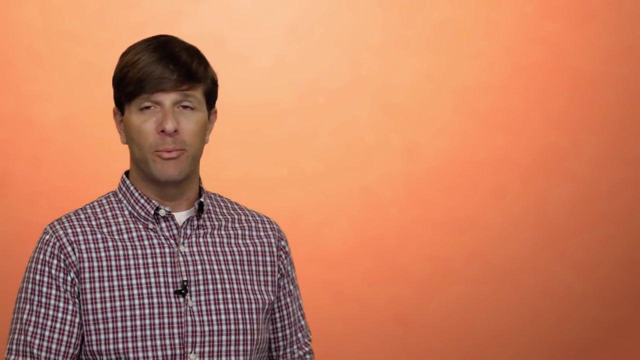 sub l times f, sub i times f, sub c times l. Now n equals the number of intelligent civilizations out there whose communications we could possibly detect within the Milky Way. In other words, it's the number of potential alien civilizations out there in the Milky Way that we could conceivably. 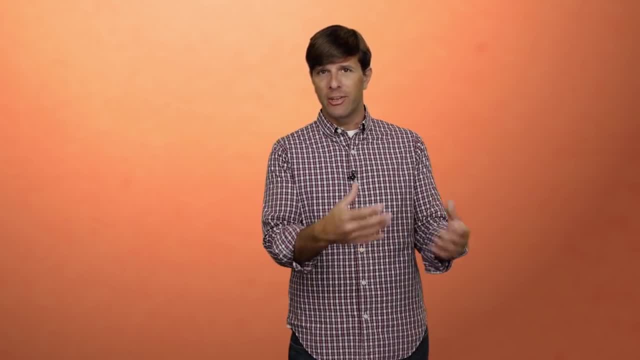 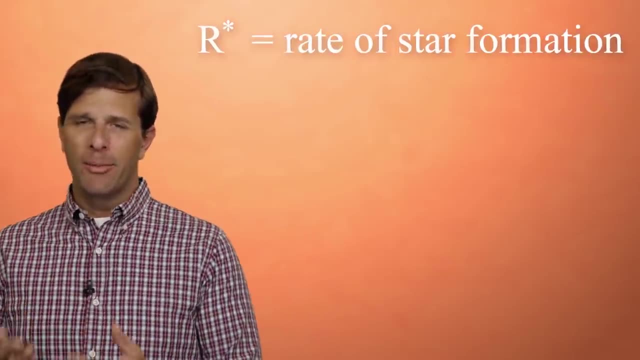 interact with. This is the point of the Drake equation. It's what it seeks to understand Now. r star is the rate of star formation. Astrophysicists have determined that in the Milky Way about three solar masses worth of material forms into stars every year. Now, solar mass 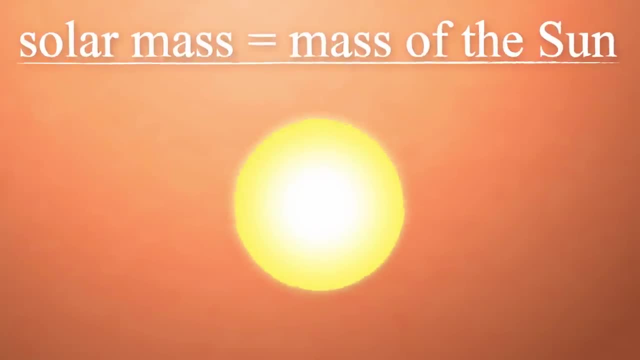 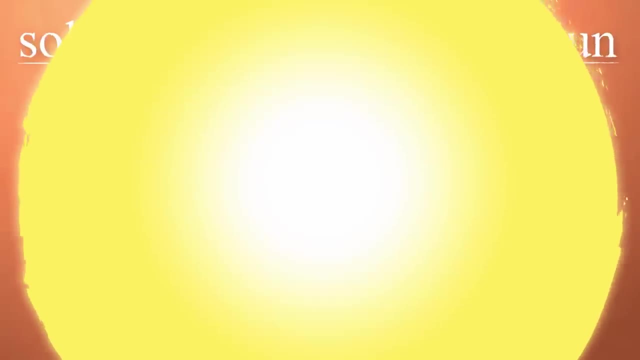 is equal to the mass of our sun, And three times that doesn't necessarily mean that three suns are made. It could be one massive star that's three times the mass of our sun that forms that year, or it could be ten smaller suns that are .3 times the size of our sun. 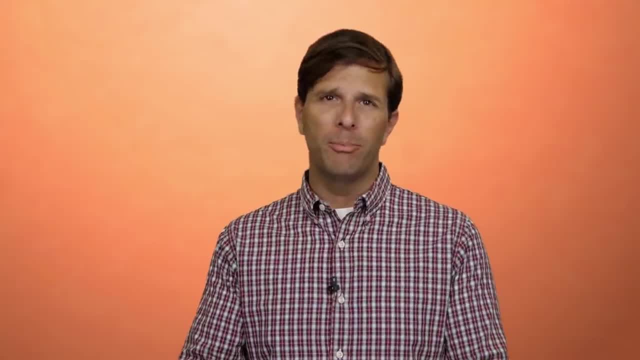 It could be any combination of those, but for our intents and purposes, because our sun is technically an average-sized star, we can say three. In fact we can say a very regular number, just for the鉵 of the sun. A very common way for us to come up with a value is to use the equation F sub p. 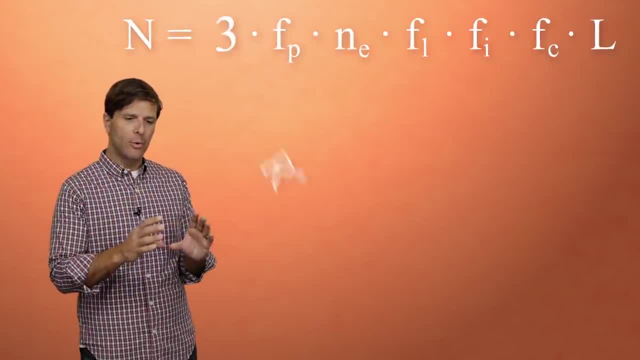 F sub p is a fraction of how many stars are orbiting the planet. but both of these stars are not cold or too hot, So we can basically use a bit of the equation to estimate how many stars are orbiting the planet. but if we could put it up to three, making eight of them our stars, we get three. 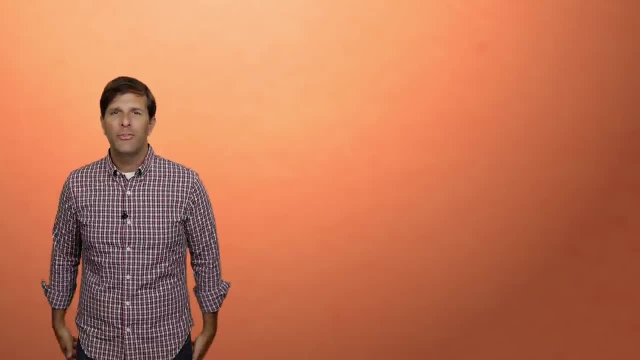 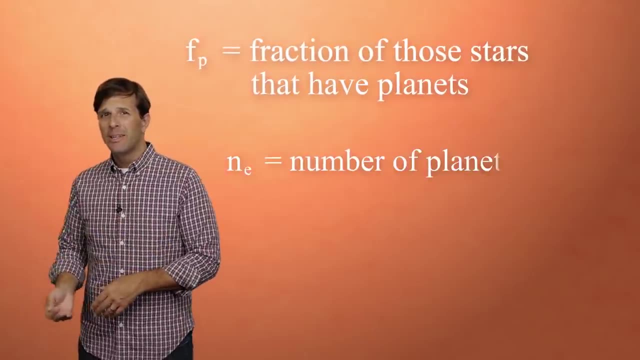 and we arrive at what is to be a very rare occurrence where we have a value that we can put in pretty confidently into the Drake equation. F sub p stands for the fraction of those stars that have planets orbiting them. N sub e stands for the number of those planets that are capable of supporting life planets. 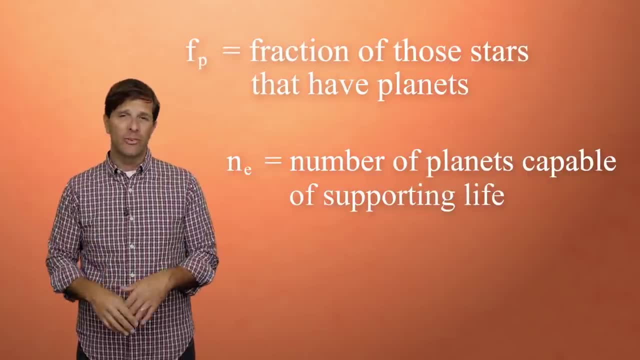 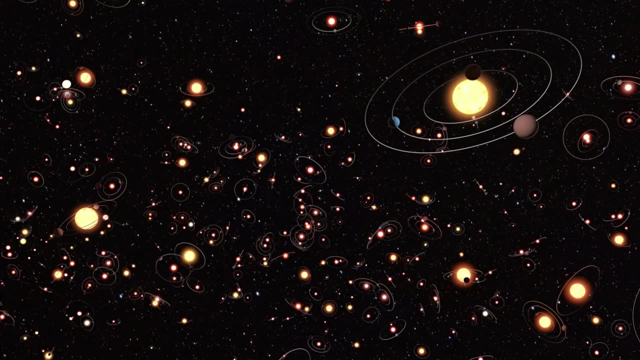 that orbit the star within its Goldilocks zone, where things are not too hot or not too cold, but just right. but just right. We call these exoplanets and we've been discovering them like crazy lately. There could be possibly billions in the Milky Way alone, but so 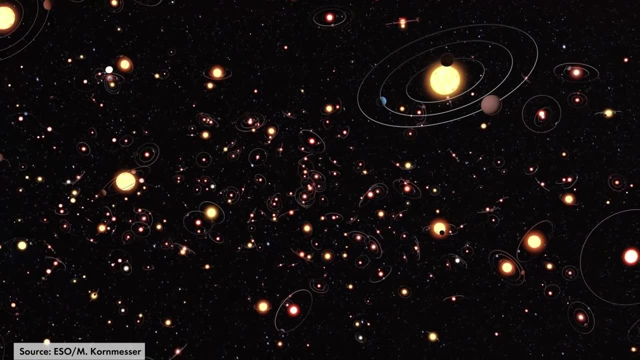 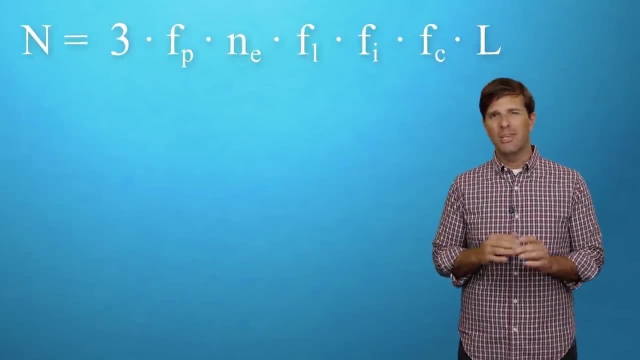 far, we're pretty confident that there's at least 3,400 exoplanets or planets capable of supporting life within the Milky Way. We arrive at the other value that we can fairly confidently put into the Drake equation: 3,400.. From here on, 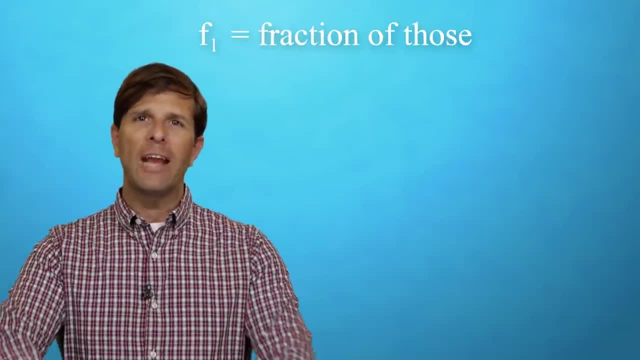 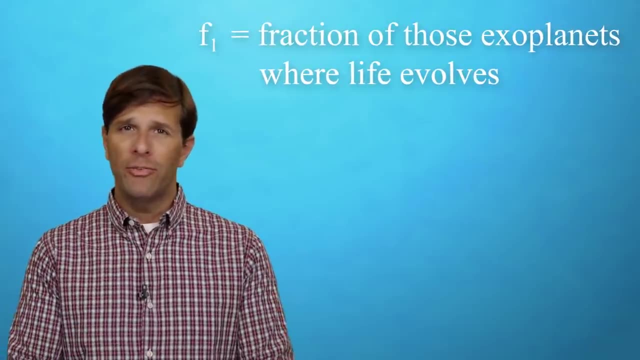 out, though it gets increasingly murky. F sub L stands for the fraction of those exoplanets where life evolves. So far we can only say with absolute certainty that life has evolved once in the universe. and since we're talking about ourselves, we can't really input one into the Drake equation because we're not. 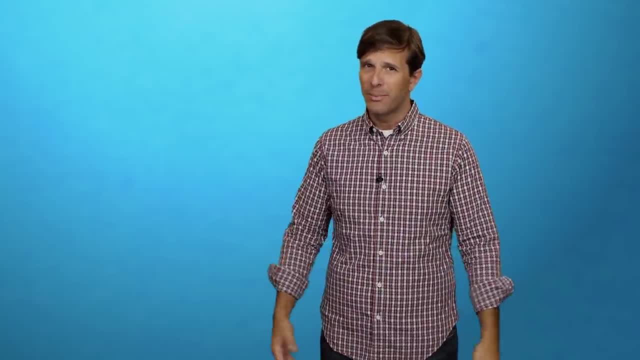 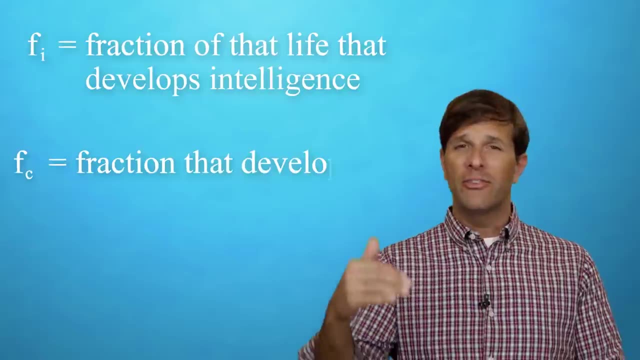 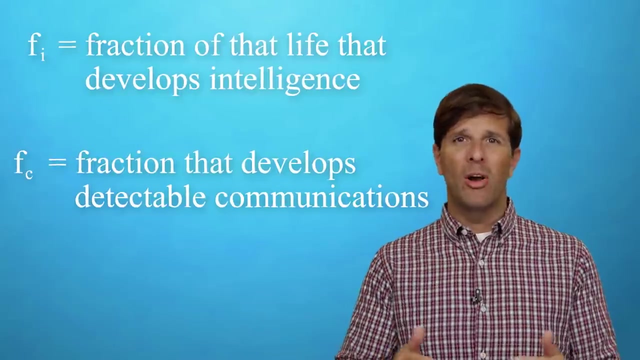 seeking to find out whether we can communicate with ourselves or not. you know what I mean: F sub I is the fraction of that life that evolves, that develops intelligence, and then F sub C is the fraction of that intelligent life that develops communications, that transmits in ways we could detect, basically along 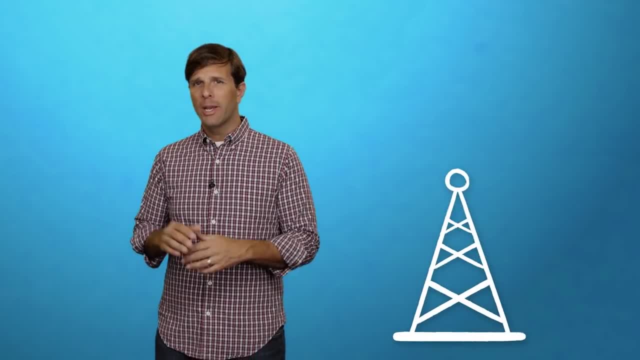 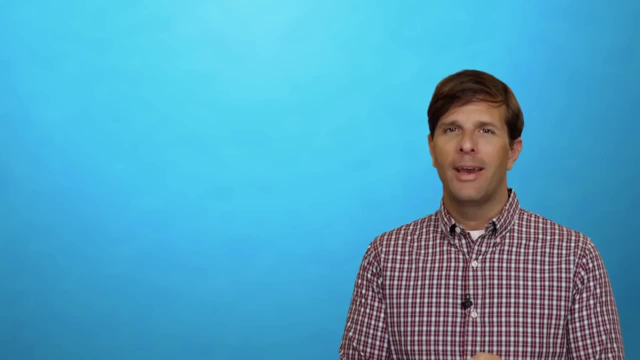 the electric field, Electromagnetic spectrum, In other words, it's kind of like what kind of chatter boxes are out there using radio waves, like we are with, like I Love Lucy, blasting through space still? And then finally, L, the big L, stands for the. 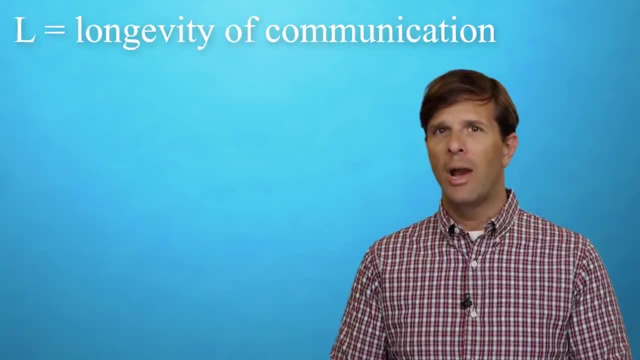 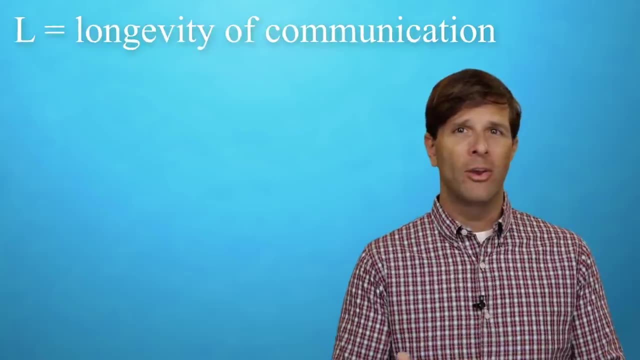 longevity of this communicativeness, right? So how long does the average intelligent civilization transmit in some way that we can detect, before they either go extinct or find a new means of communicating that we couldn't possibly detect, like, I don't know, telepathy? So, as you can see, when you put all that, 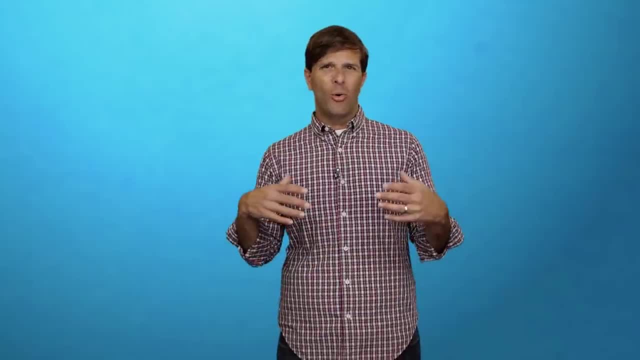 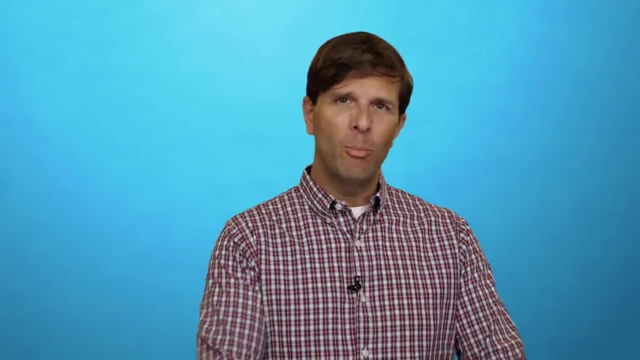 stuff in together. the Drake's equation doesn't really tell us a whole lot about how probable it is that there's intelligent life out there in the Milky Way. But it's not the Drake equation's fault. don't blame it, stop, stop Instead. 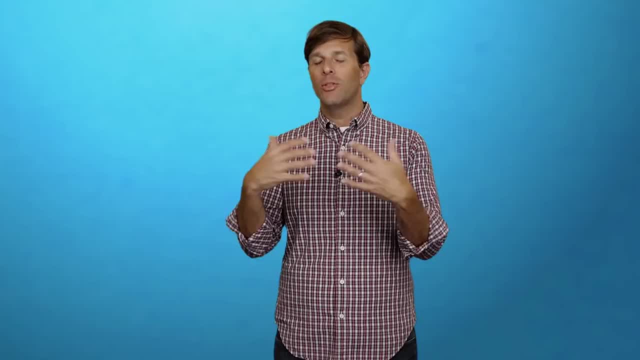 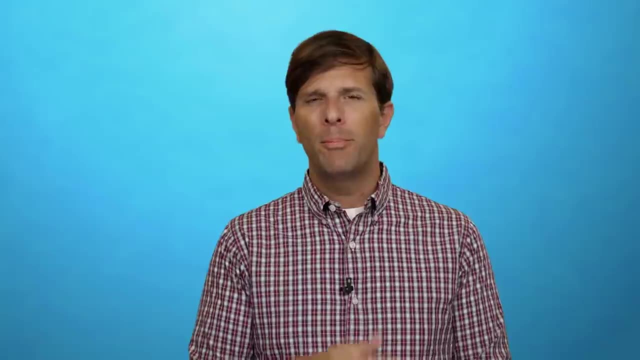 it's because we don't understand the universe, we don't understand the Milky Way, even we don't even understand life well enough to really confidently put some good, educated guesses in there. The problem with the Drake equation, though, is that not only can you prove that there's a really high certainty, depending 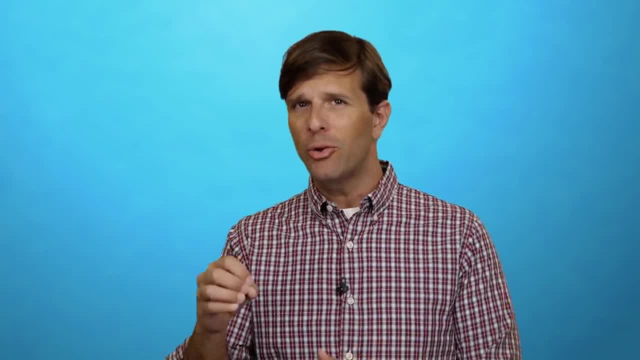 on what wild guess you put in there. but it's not the same as the Drake equation. You can also prove that there's a zero chance. All you have to do is put zero into any one of those factors and the possibility that there's any life out. 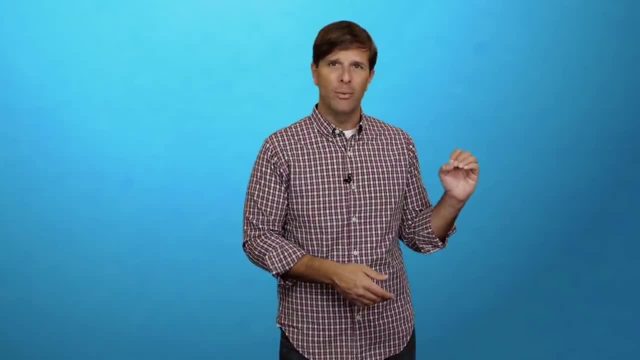 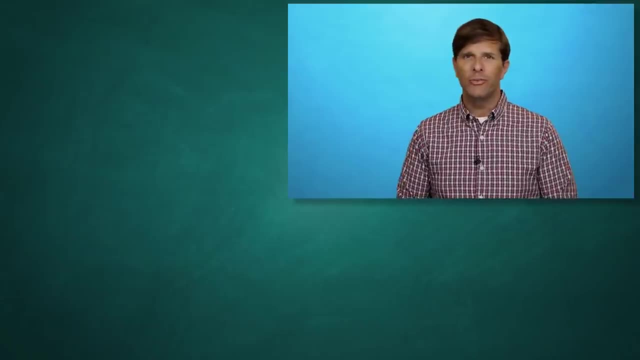 there that we could possibly detect or communicate with is zero. It's a problem. So astrobiologists and astrophysicists and astronomers will keep searching the universe, will keep searching the Milky Way, and the data they come back with will be plugged by some people into the Drake equation to see if it will. 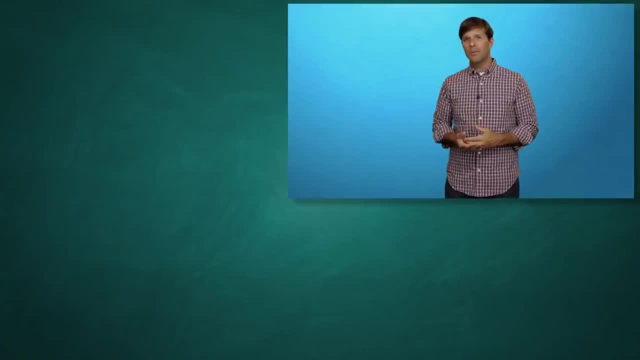 eventually spit out a verifiable answer, But in the meantime it's serving as a pretty great tool for getting people to think about the possibility of alien lives, and not just that, but about the future of our own human civilization as well.